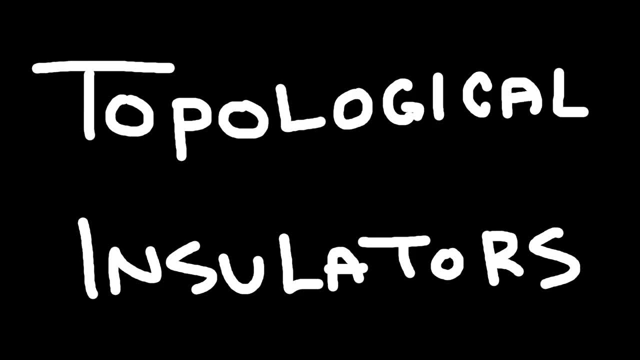 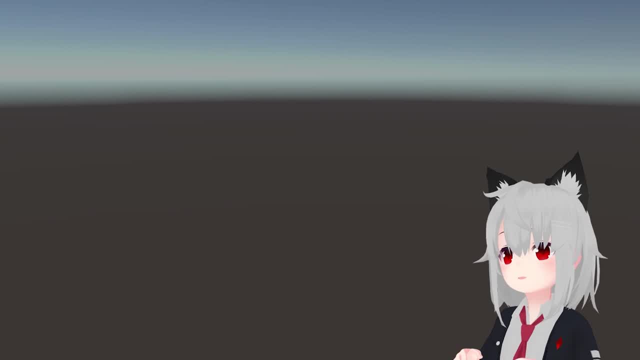 Hey guys, so today I'm going to talk about topological insulators. These are a class of electrical insulators in condensed matter physics, whose mathematical underpinning turns out to have a lot to do with the field of, well, topology. Here one studies equivalency classes of objects. 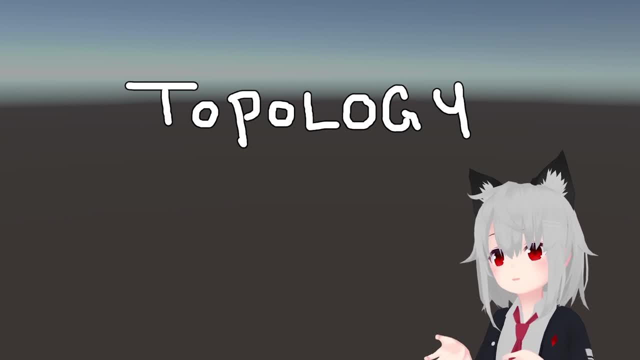 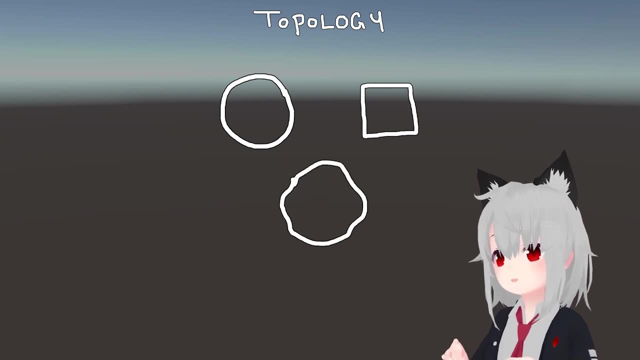 based on the presence or absence of continuous deformations between them. You can think of, for example, the circle and the square. In this case, it's straightforward to see that there exists a continuous deformation between them, so that they're said to be topologically equivalent. 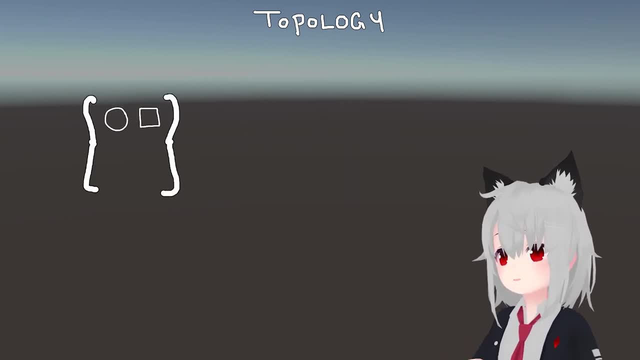 and that they belong to the same topological equivalency class. The triangle also belongs to this equivalency class. so does the hexagon or any 2D shape, really, since they can all be continuously deformed into each other. Well, are there shapes which these can't be continuously? 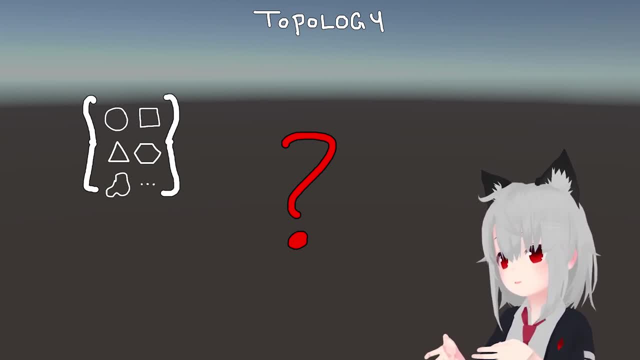 deformed into. Are there other distinct topological equivalency classes? The answer to that question turns out to depend on the details of the topological space. In our case, let's assume that there's a hole in the topological space and let's draw a circle. 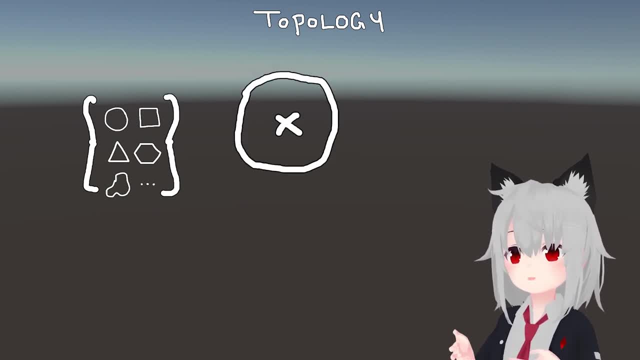 around that hole. Now this circle can still be continuously deformed into a square or any other 2D shape which also has a hole in its center. The problem arises when you try continuously deforming these shapes into shapes which don't have holes in their centers, since there is no 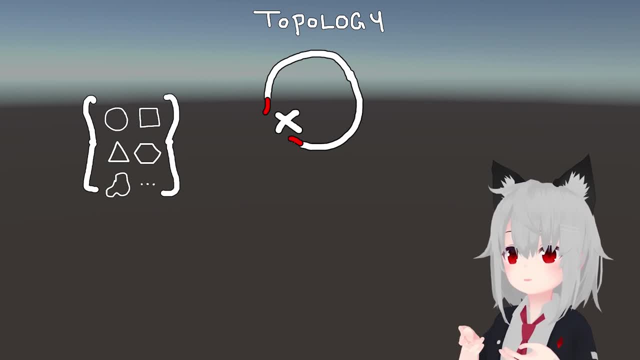 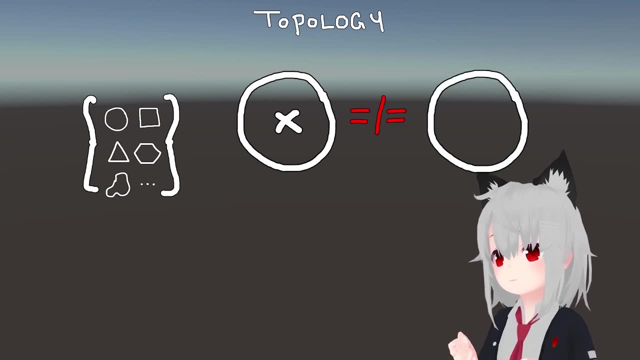 way to do this really without ripping or tearing, something which would correspond to a discontinuous transformation. For this reason, shapes with holes in their centers are not able to deform into shapes that are typically distinct and that they belong to a distinct topological equivalency. 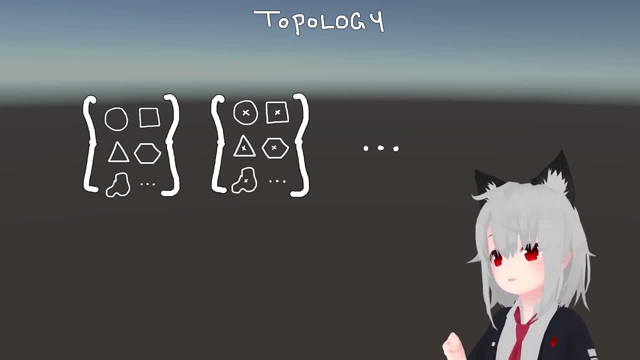 class. Now you can repeat this procedure for 2 or 3 or an infinite number of holes, ultimately giving you a set whose elements are characterized by an integer representing the number of holes inside the shapes. Now this integer is called the topological invariant of the. 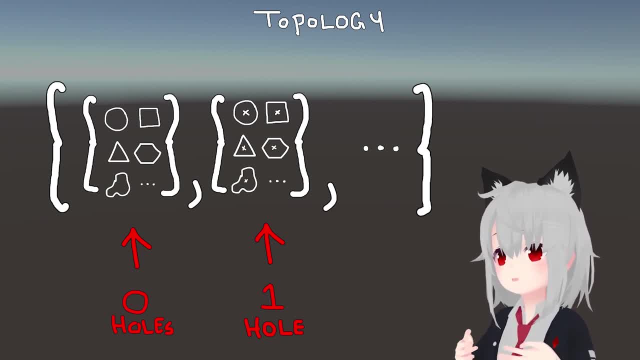 shapes, and it can be shown quite generally that there always exists a bijective mapping between the set spanned by this topological invariant, in our case the integers, and the set of topological equivalency classes. For this reason, you're free to think. 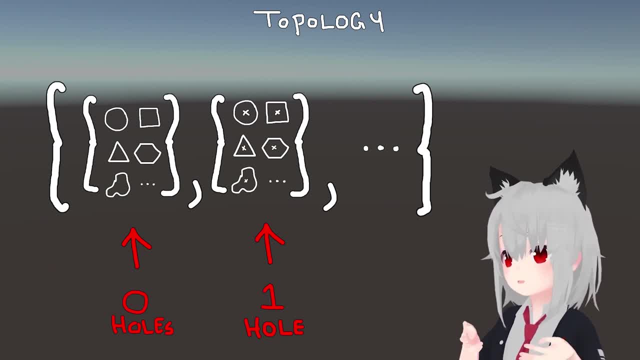 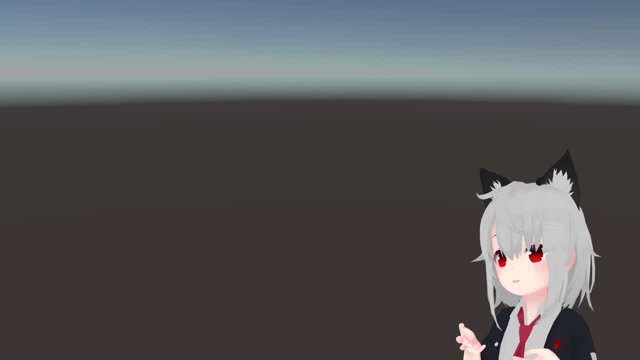 either in terms of the topological invariant itself or, equivalently, in terms of the shapes that it represents. Okay, so this is pretty cool, but what does it have to do with physics? Well, remember that we're talking about condensed matter physics, not just physics generally. 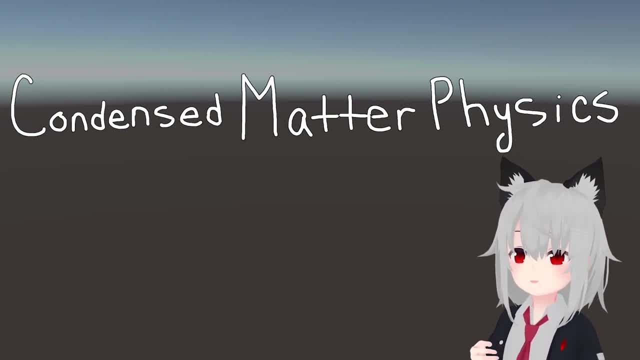 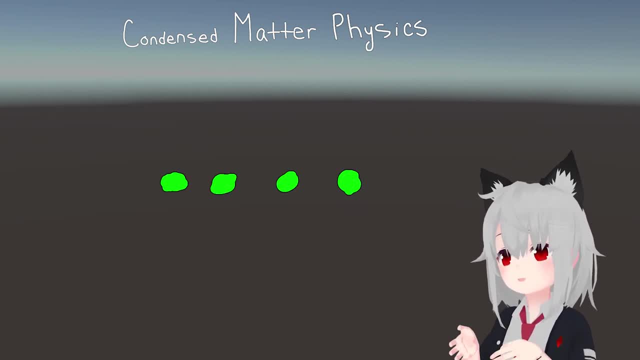 A surveillance device is a covered glass trap to develop a vision like the image of a boy or me taking a look around the nowhere system in a main square. Let's basically go ahead and Zhu Yiling and check it out. Ou, child based IELTS. 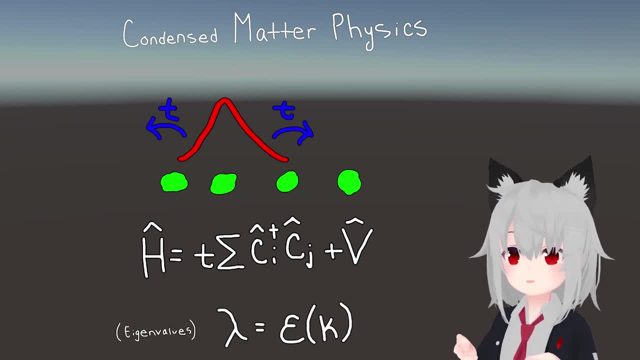 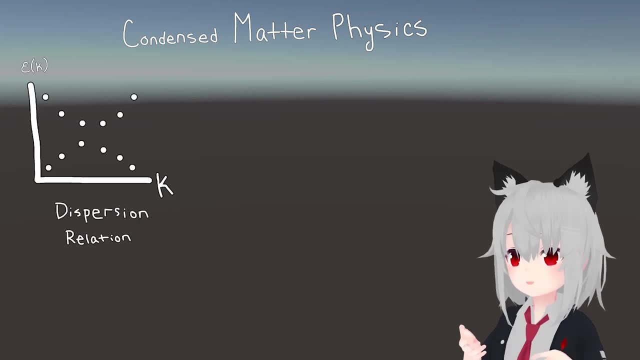 них, You have the following results: say, momentum. Now, if you plot out the energy levels, you'll get a dispersion relation which will exhibit a discretization of the energy levels as a result of the quantum Hamiltonian that we started with. However, if you assume that the length of the system is much, much larger than 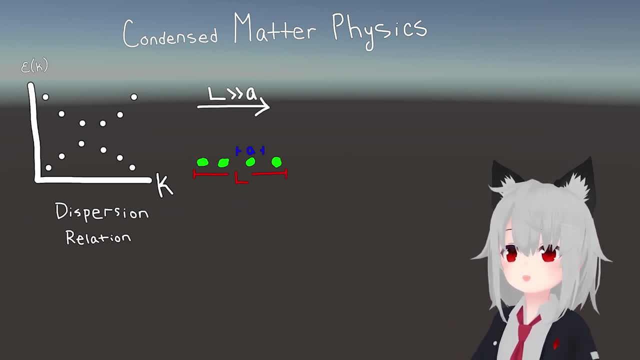 the typical interatomic spacing, as it usually is. then the spacing between consecutive momentum values, which goes like one over the length, becomes so small that you can basically approximate this dispersion as a continuous function called the band structure. This band structure is basically a visual representation of what the allowed quantum states are as a function of momentum. 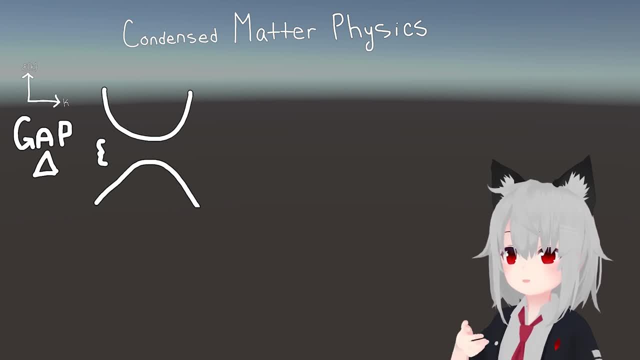 Now, this band structure may or may not have a gap at some point, but if it does, then this turns out to have important ramifications on the transfer properties of the material. To understand why, let me first define something called the Fermi level as the energy at which the highest energy 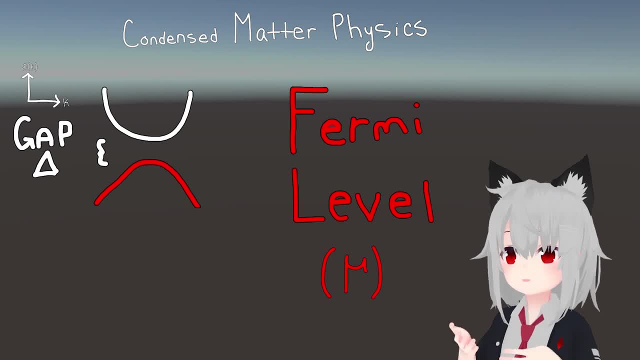 electron exists. You can think of grads of temperature in the form of a number of electrons and an energy at which the highest energy electron exists. You can think of grads of filling up the band structure with electrons. The last electron to enter the band structure lies at the Fermi level. Now let's place our Fermi level inside. 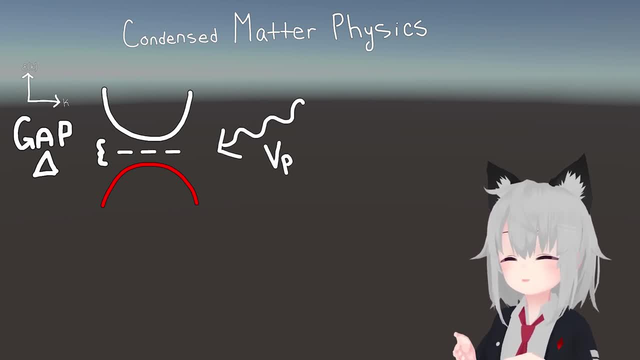 the gap and let's think about perturbing the system with some characteristic energy scale. If the magnitude of the gap is much larger than this characteristic energy scale, then there's a sense in which the electron simply won't respond to the perturbation because it's not giving them enough energy to jump the. 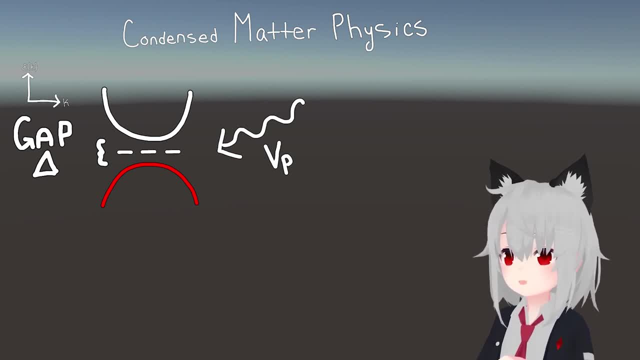 gap and reach the next available quantum energy state. This results in electrically insulating behavior, in the special case of the perturbation corresponding to an applied voltage bias and the response being the motion of the electrons. Now, the opposite end of this extreme is, of course, the gapless case. 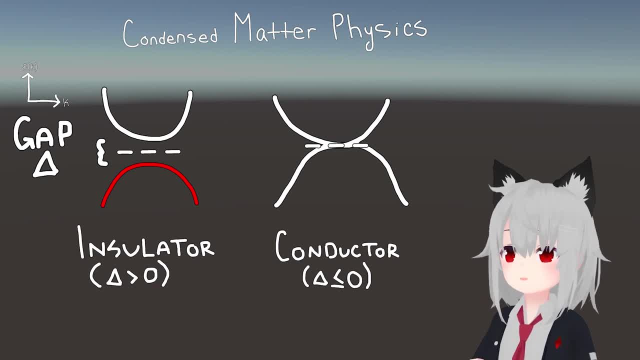 which would result in electrically conducting behavior by virtue of the fact that, for all values of the Fermi level, there's always an infinitesimally close quantum energy state for the electrons to respond with. Okay, but let's focus for the moment on the insulators. That is, after all, the purpose of the 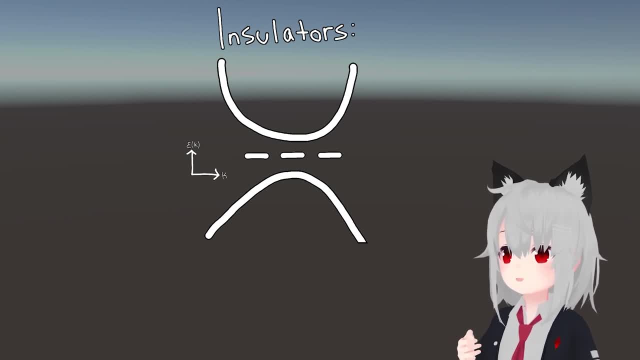 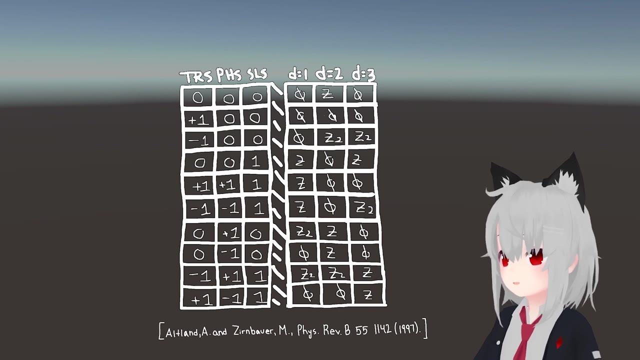 talk And let's think about things topologically. This amounts to asking: what are the topological equivalency classes associated with continuous deformations of the underlying Hamiltonian? Now the answer to this question turns out to be not so obvious, but researchers have shown that you can. 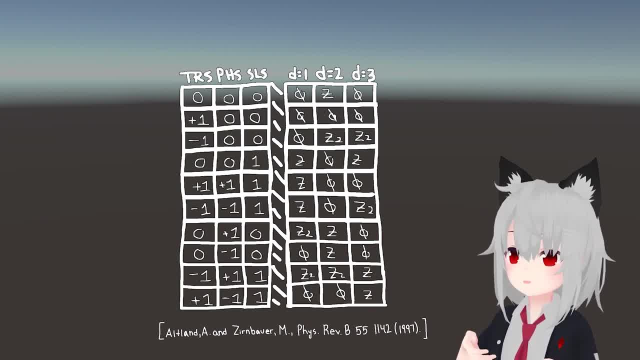 get some idea about the nature of the topological invariant, assuming you know some basic information about the insulator, in particular its dimensionality, along with the presence or absence of time-reversal symmetry which takes time to minus itself. particle-hole symmetry which exchanges filled and empty states. 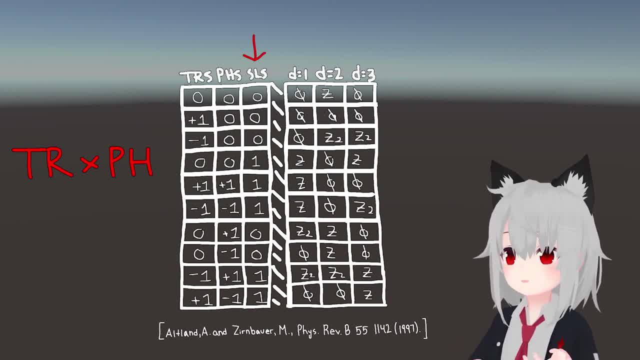 and sublattice symmetry, which is defined as the composition of the prior two operations. With this, you can determine whether your topological invariant is an element of the set Z2, which is the integers mod 2, whether it's an element of the trivial set, which is basically just 0,. 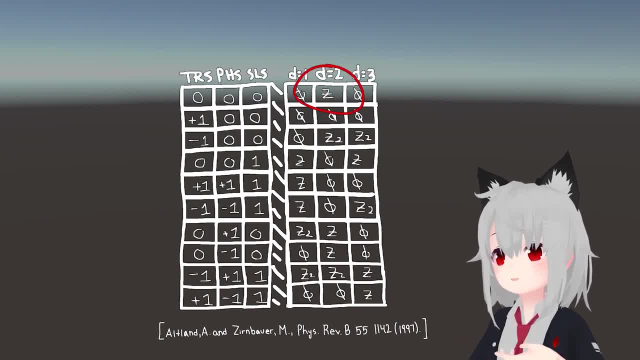 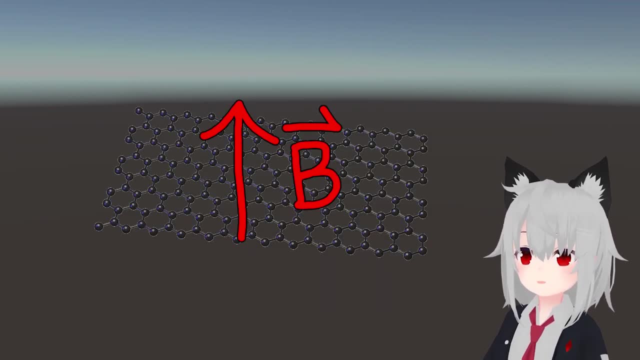 or whether it's an element of the integers, as we saw in our first example. For concreteness, I'll pick one of these classes, say a two-dimensional class which breaks time-reversal symmetry but preserves particle-hole symmetry. This might correspond to something like a monolayer of graphene in an externally applied magnetic field. 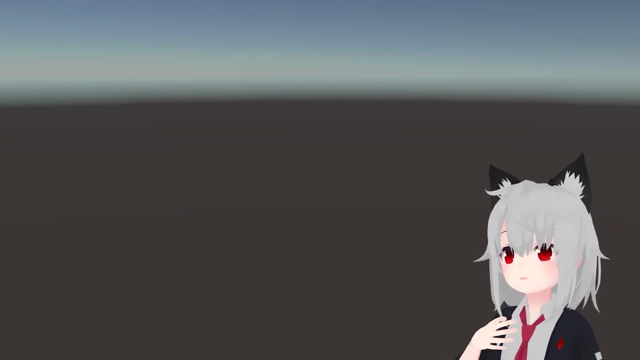 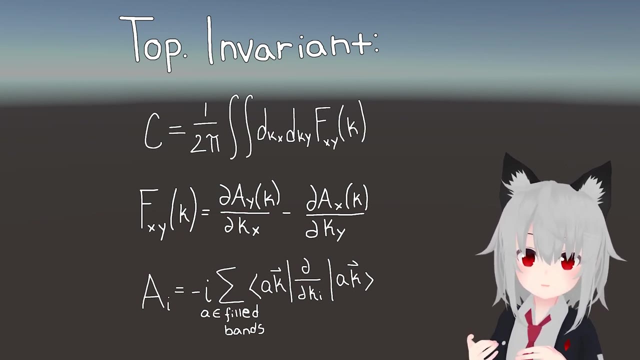 but in any case, the topological invariant in this system can be written down as the Chern number, which is physically defined as the integral of the Berry curvature over momentum space. Now, this Berry Curvature is interesting in its own right and definitely worth looking into. 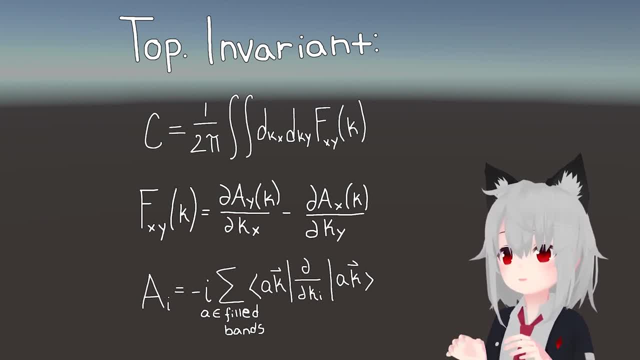 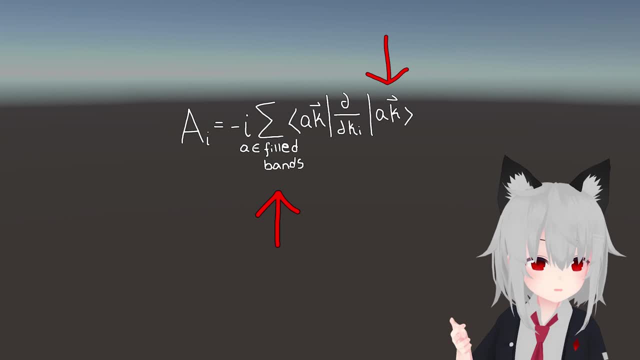 But for our purposes, all we really need to know is that this topological invariant depends on two things: The first is the number of filled states and the second is the mathematical structure of those filled states. Now we will only be concerned with adiabatic transformations, which are defined as transformations which do preserve their structure. 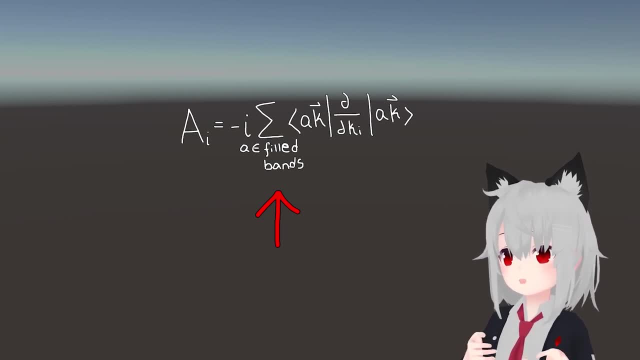 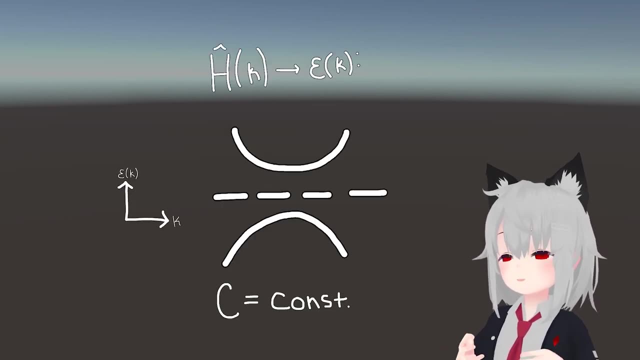 So we're really only left with one thing, which is the number of filled states. What this means is that if we want to maintain our topological character, embodied by the topological invariant, then we're free to deform our Hamiltonian and its underlying band structure in any way that we want. 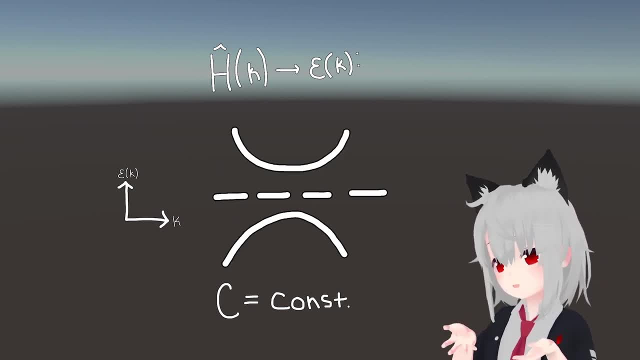 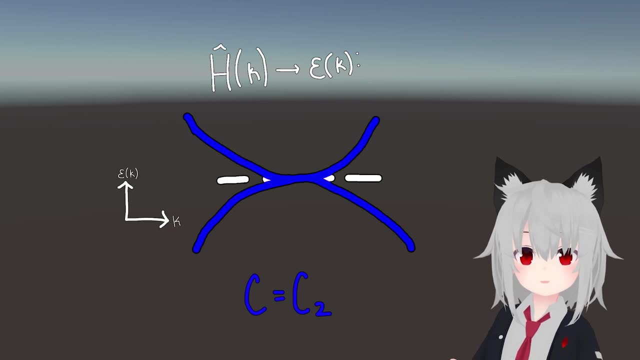 so long as we don't cross the Fermi level or, equivalently, close the gap. The converse of the statement is also true: If we do want to change our topological invariant, then we must first necessarily close the gap and then maybe reopen it. 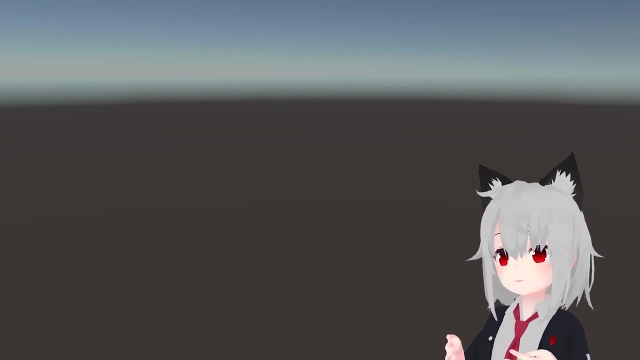 This results in one of the most awesome statements about topological insulators generally, which is the presence of gapless edge states. gapless, we know, means conducting, and edge states are just states which are localized at the edge or a boundary. In two dimensions, this would correspond to something like 1D wire states and, in three dimensions, two-dimensional surface states. 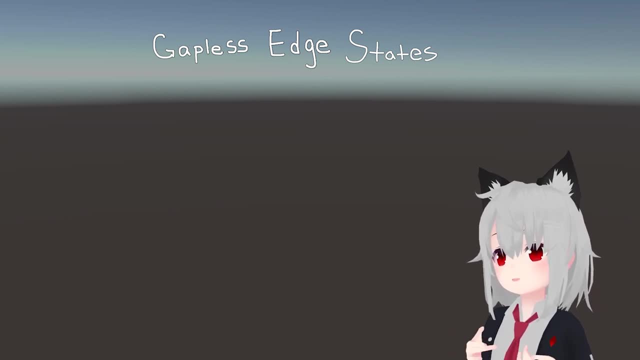 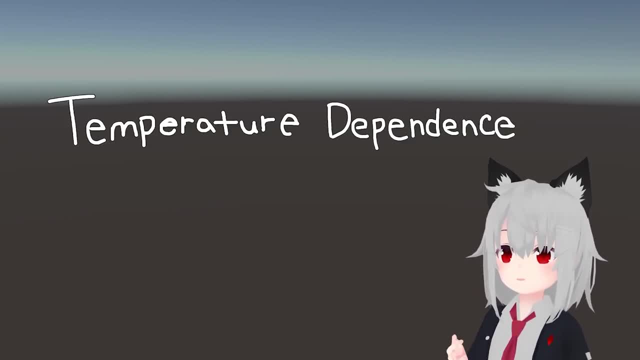 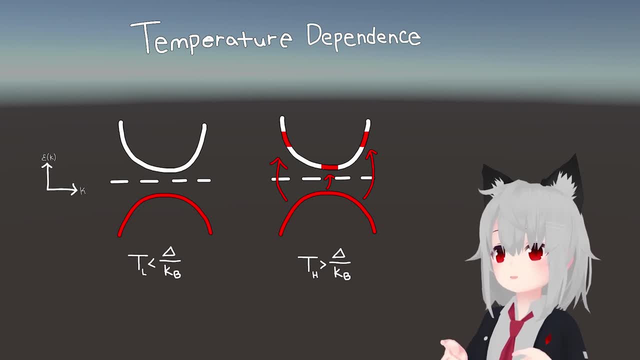 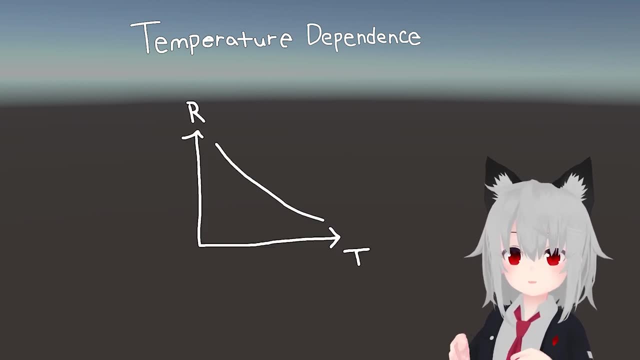 behavior, not quite insulating, but not quite conducting either. As a result, the high temperature resistance is a bit lower than the low temperature resistance, giving you a curve which would embody this. Okay, so how does this change in the presence of gapless edge states? Well, in this case, 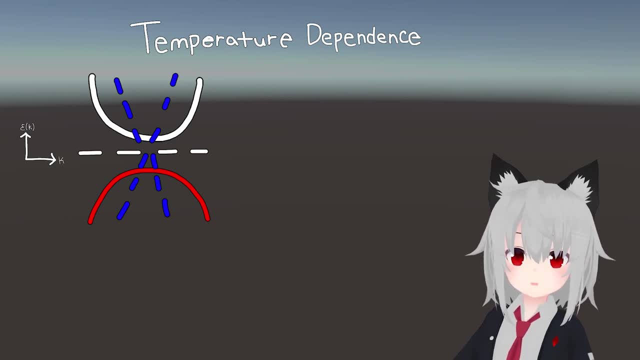 you'd have to superimpose the gapless dispersion on top of the original insulating band structure. Now it turns out that at sufficiently high temperatures this doesn't really change much, because the thermal energy kicks electrons upwards and makes them mostly interact with. 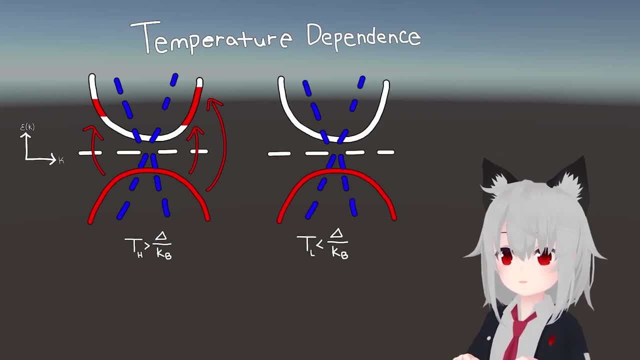 the original band structure anyways. However, at sufficiently low temperatures, the electrons are forced to live inside the gap, and now you have a gapless dispersion which provides an additional mode for conduction which shouldn't really have ever been there in the first place. 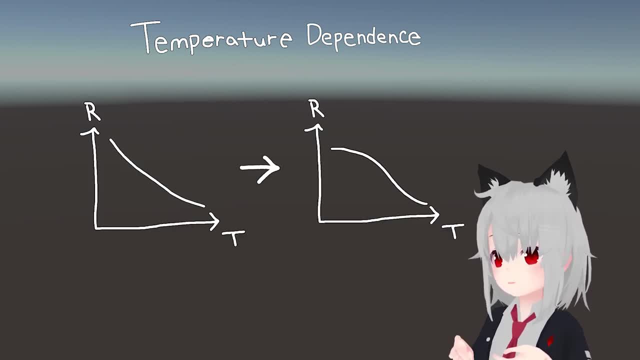 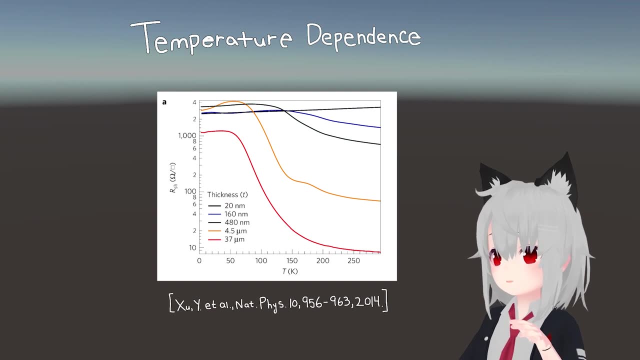 This results in a net reduction of the measured resistance at sufficiently low temperatures and a modification to the curve that can be measured. In fact, this is exactly what was measured in the prototypical topological insulator bismuth selenide, So that's already one hint at the existence. 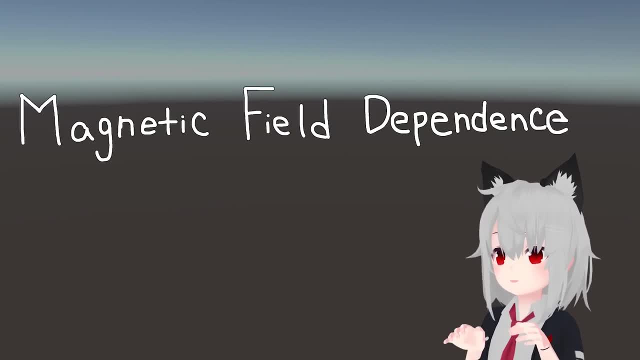 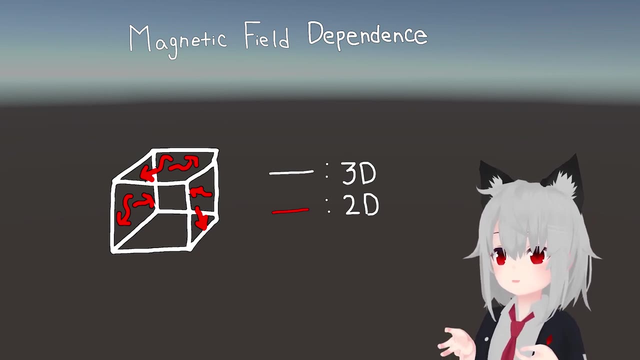 of gapless edge states. In this case, instead of exploiting the band structure of the system, we can think simply in terms of its dimensionality. In particular, if you have a three-dimensional topological insulator, then you should have two-dimensional gapless edge states, so that we can ask what. 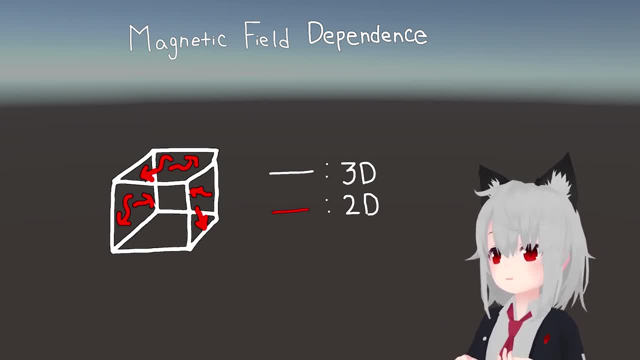 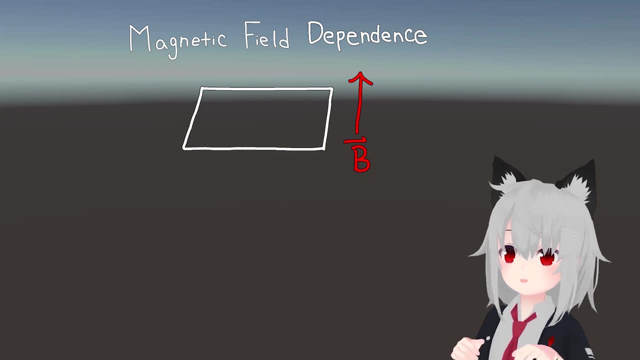 if any, are the unique features of two-dimensional electrons exposed to a magnetic field? Well, if the magnetic field is perpendicular to the two-dimensional plane, then this should induce a gap In the quantum regime. the energies associated with these orbits are, of course, quantized. 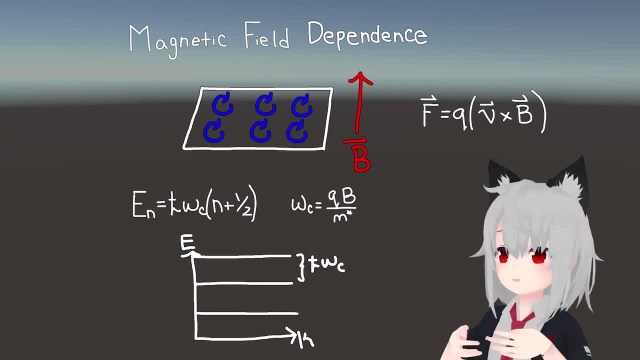 giving you a dispersion relation whose energy levels are all spaced apart with a spacing that depends on the strength of the magnetic field. This is basically a gap system, and if the Fermi level lies inside one of these gaps, then you'll get a highly resistive